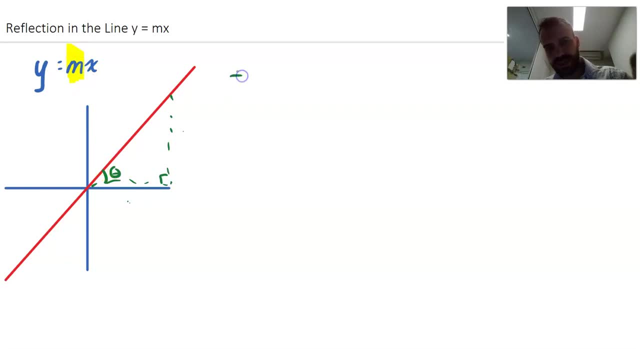 and this is the opposite here- windows of the gradient as tan theta, because tan theta equals opposite over adjacent, equals rise over run. m equals rise over run. tan theta equals rise, hold on. So it's going to be very important for us to understand that y equals mx is actually y equals. tan theta. I'll put the x on the back. Y equals X, tan theta, while you think this sound very much funny to me, so we might change this up. y equals x Shan, not the one that's come to the table here. x will be reflected. so to who use? because you know X mostly more bounce is. the problem is that. 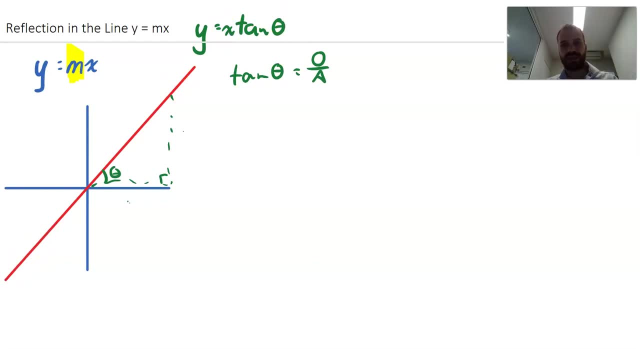 the problem is the feedback, the平 aspect of the хороший. very similar proof that the See. we can maybe use some of this blue straight forward direction randomства: y equals x. asheus tan theta. Tan theta is m, m is tan theta, which now means that we can think about our y equals mx. 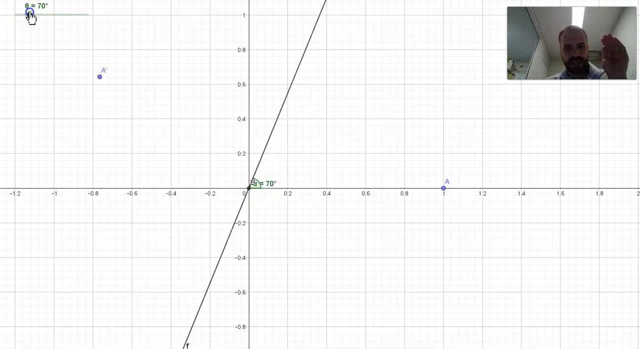 in terms of this little angle here, and as I change my y equals mx, as I change my angle there, you can see that line moves and our reflection moves as well. Now I talked about the reflection as a rotation. you can see as the line changes. so to the circle, it rotates. it's rotating around a. 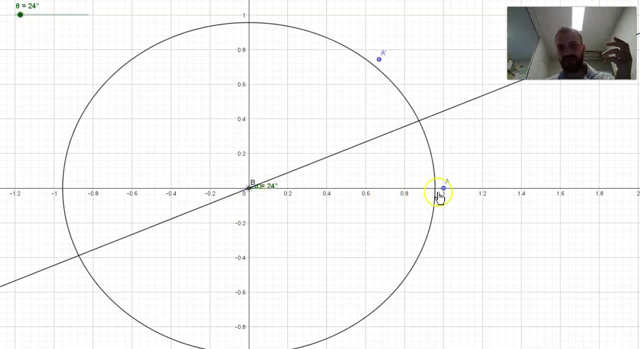 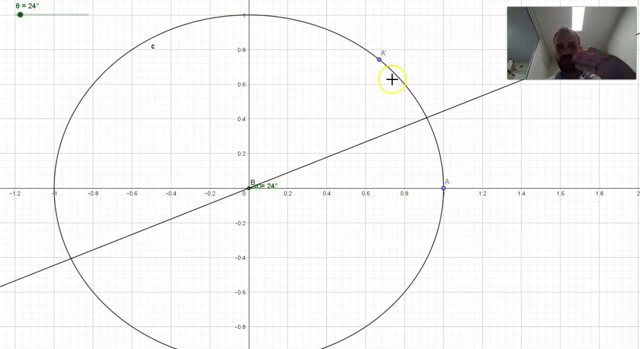 circle and a specific type of circle that you've already met: the unit circle. So this, as we reflect in this, y equals mx. as the value of theta increases, we are rotating around that circle. All right, let's draw some pictures on this thing Now. you should already recall that the coordinates 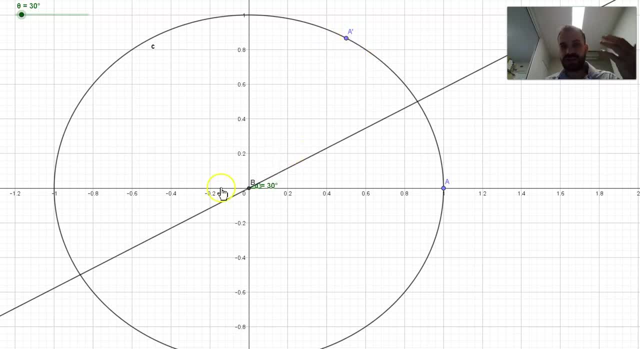 of that dot are cos theta sine theta, And I'll just draw in a little triangle so we can see that. All right, so look at this triangle here. and we said the coordinates of a dot on the unit circle are cos theta sine theta. Now cos theta? 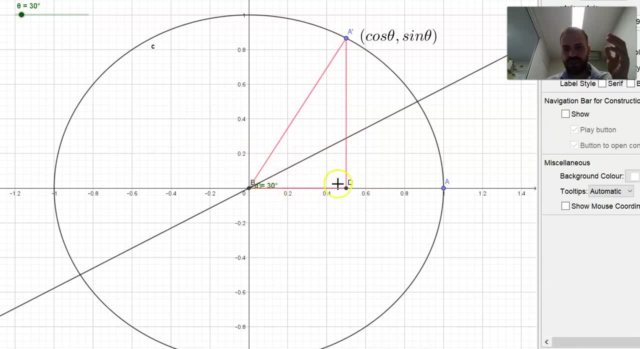 because this length here is the adjacent side of this triangle and, sine theta, because this length here is the opposite side. Now, I'm only telling half the story here, exactly half, because, look, this is our angle, theta, and it's not the full angle of the triangle, it's only. 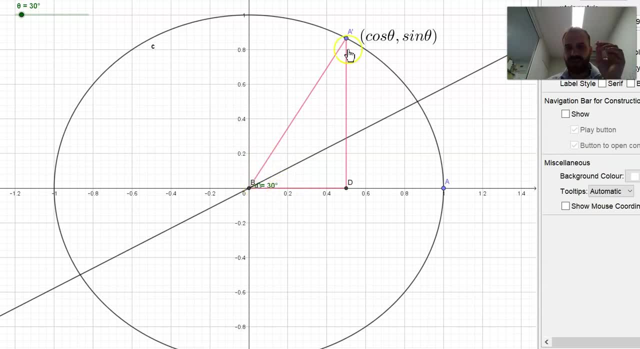 half of the angle of the triangle. So if we're going to talk about this coordinate in terms of theta, which this angle is, then this coordinate isn't theta, it's 2 theta. it's twice as much as whatever that is, and you can see as I change that angle, that remains true. 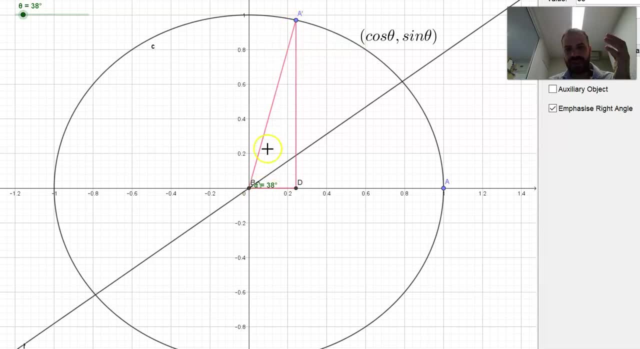 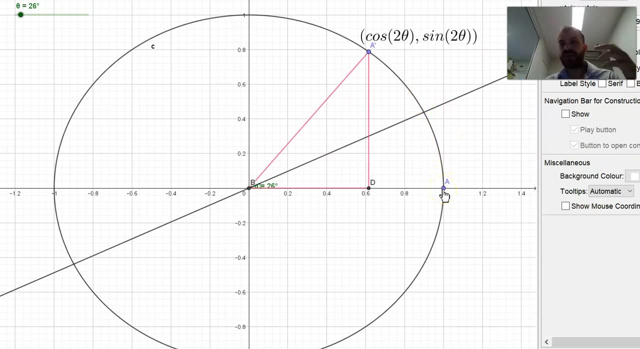 So 38 here, we're up to like 76 there. So all of that is to say that our point 0 will transformed or be transformed, to cos 2 theta, sine 2 theta, and we're going to use that as in our reflection matrix. The other point that we care about a lot is this point here: 1: 0.. 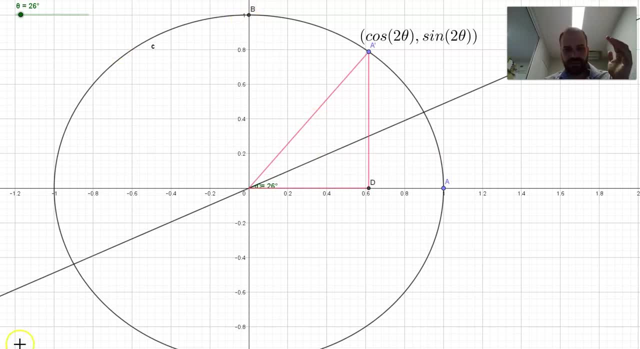 What happens when we reflect that in this, in this line. All right, it's all the way down there. you can see. Now let's try drawing in the same kind of triangle that we've got for this one. Now we can go through a proof that these two triangles are. 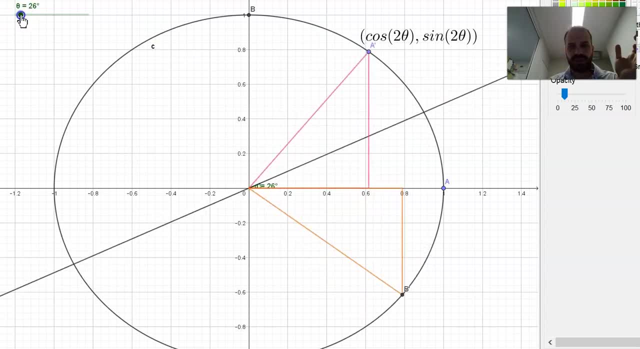 congruent. but it's going to be enough for me at the moment that we eyeball them and say what they look the same. You can see, the coordinates of of that dot are matching up with the coordinates of that dot, except reversed. Now that's got some interesting implications, because the angle 2 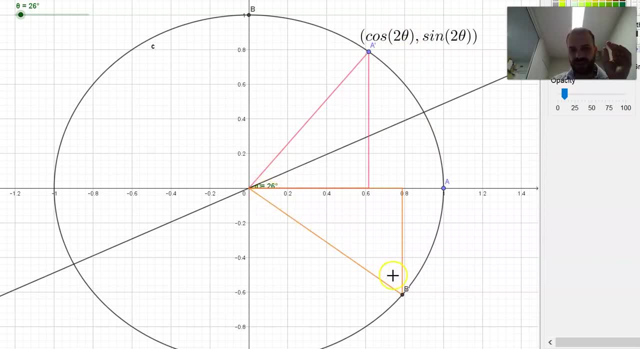 theta is not sitting here. it's sitting here Now. if the angle 2 theta is sitting there, that means that the coordinates of this triangle are not the same. So we're going to go through a proof that these dots are not cos 2 theta, sine 2 theta. They're going to be the the opposite of that. 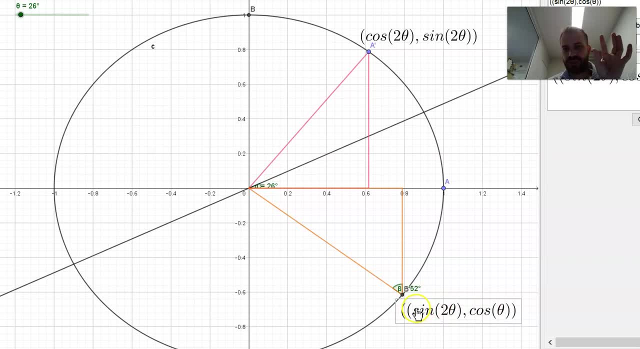 Now, that's almost correct, but let's just jump through it in turn. Sine, 2 theta is the x coordinate, which in this case is positive, so that makes sense. but cos- that should be 2 theta. cos 2 theta is negative, So we're going to need a negative in there, and now we have this fantastic. 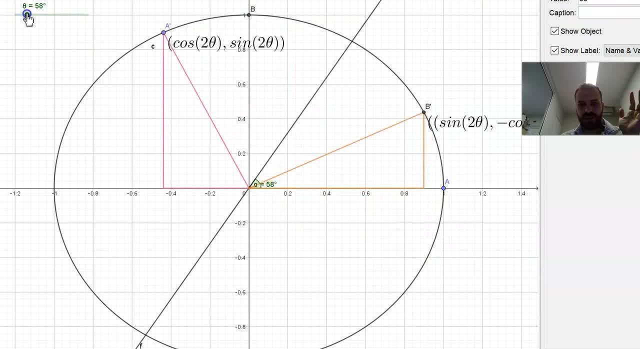 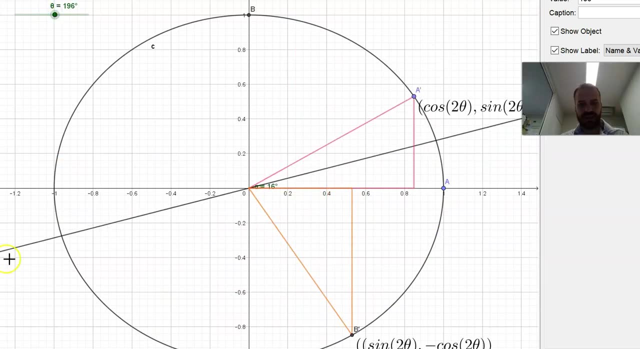 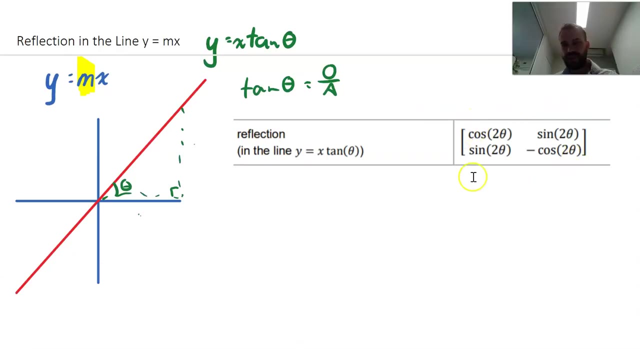 thing where we can reflect and doesn't No matter what y equals mx is. we get this cool thing going on. Okay, so that is reflecting in y equals mx. Now, practically for us, what does that mean? It means we use this transformation matrix to transform our points. So you should remember. this is the little drawing we just made.